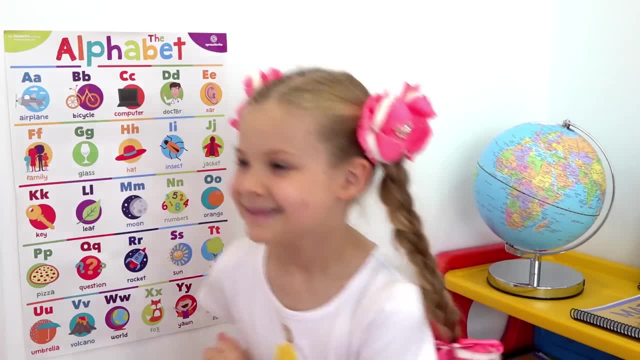 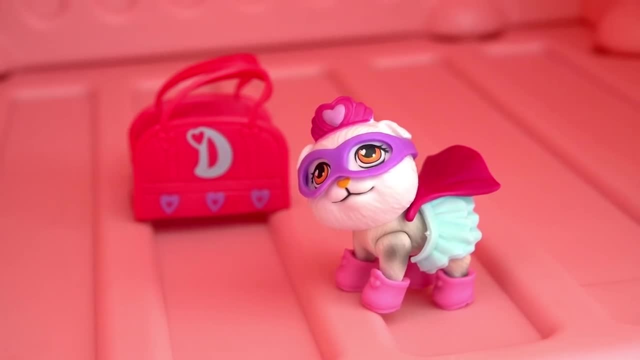 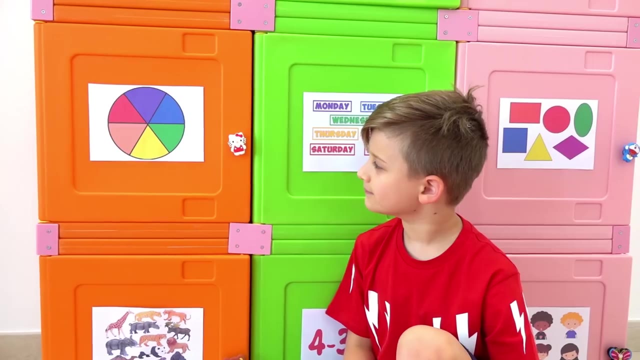 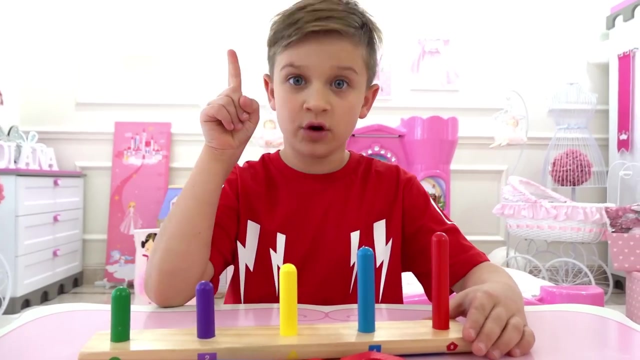 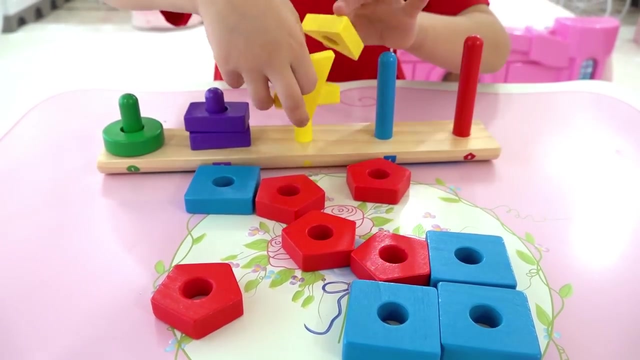 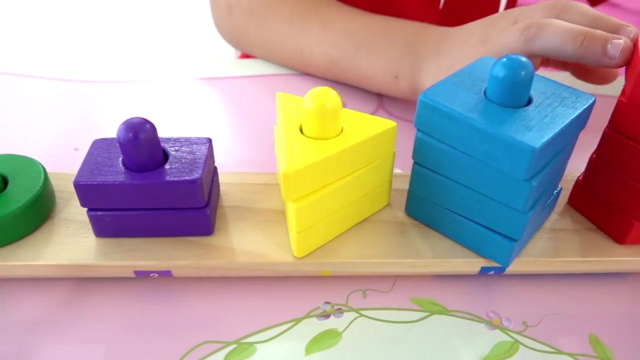 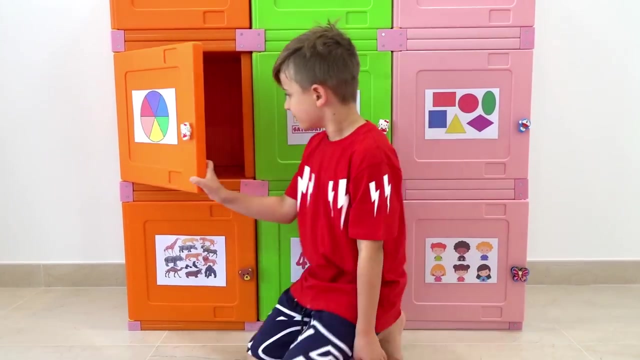 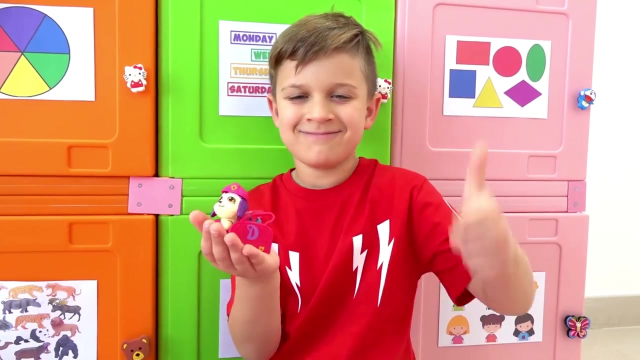 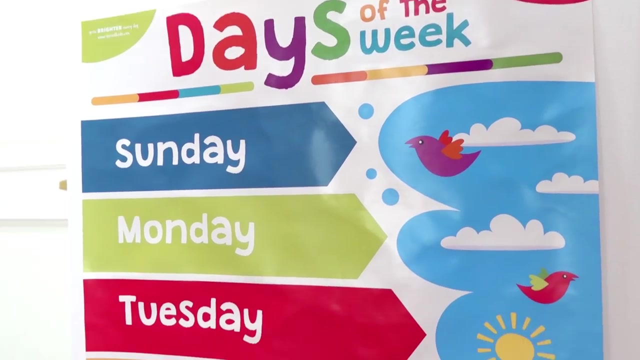 Now I know my ABC's. next time won't you sing with me? Awww, I'll save you Colors First: green, Purple, Yellow, Blue, Red, Yellow, Green, stone. Days of the week: Sunday, Monday, Tuesday, Wednesday, Thursday, Friday, Saturday, Sunday. 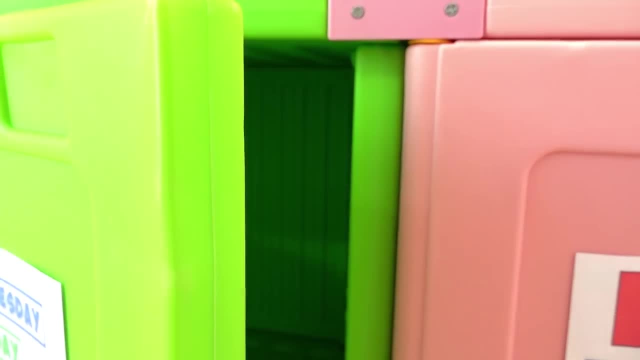 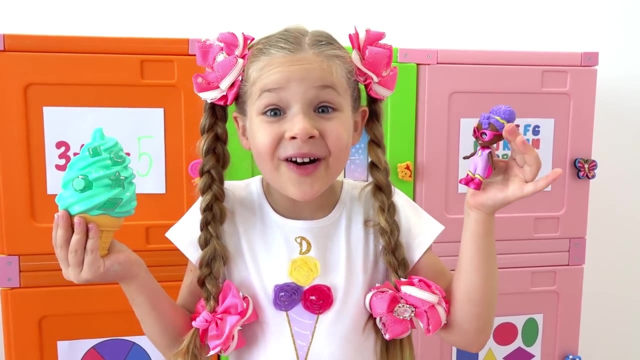 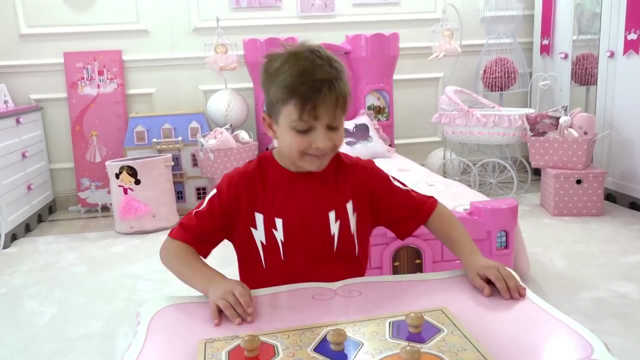 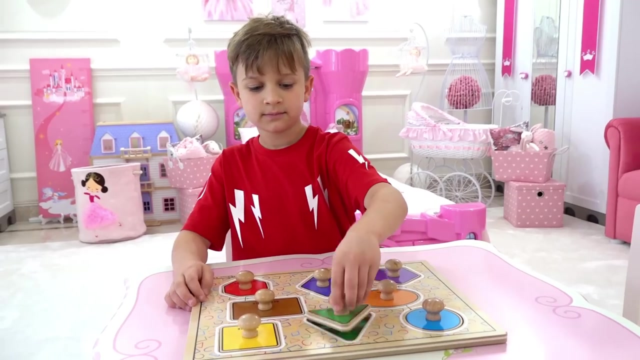 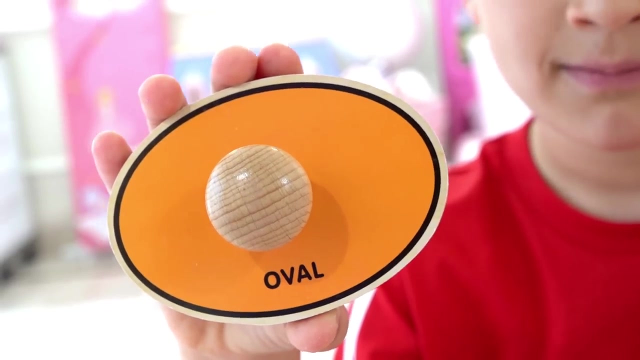 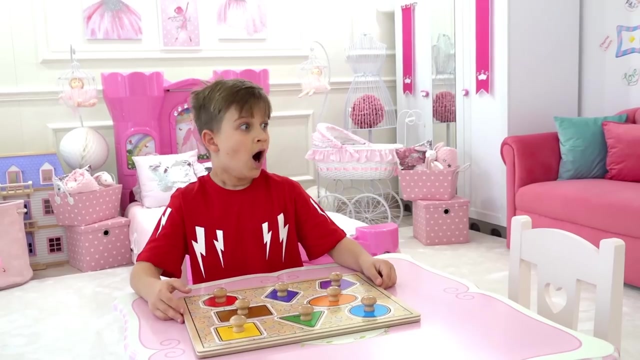 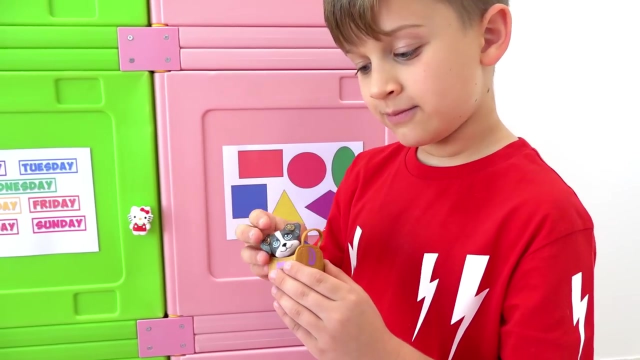 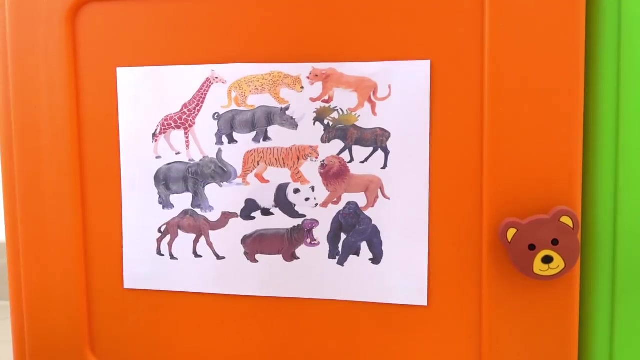 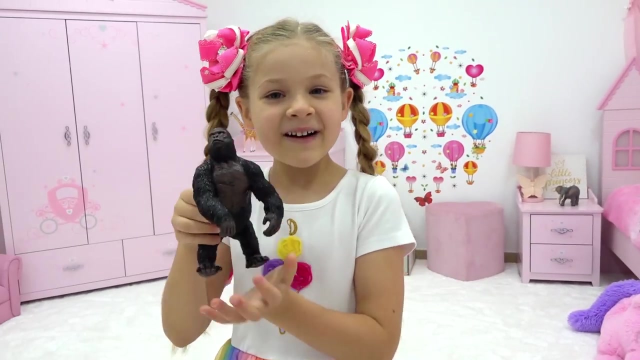 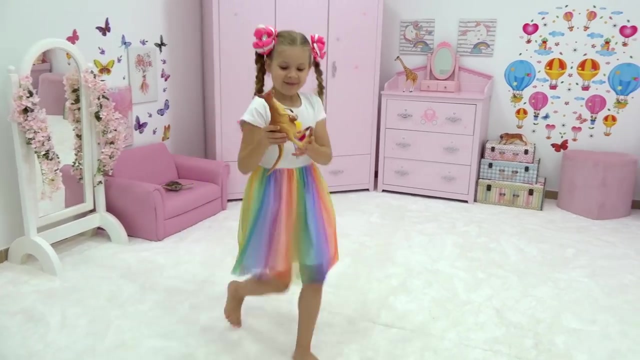 Friday, Saturday, Saturday day. Wow, Super hero Shapes. Let's learn the shapes: Circle, Triangle, Square, pentagon, oval, rectangle, diamond, octagon. oh, puppy, i'll save you. animals. let's find animals. i know: gorilla, crocodile, kangaroo and baby. 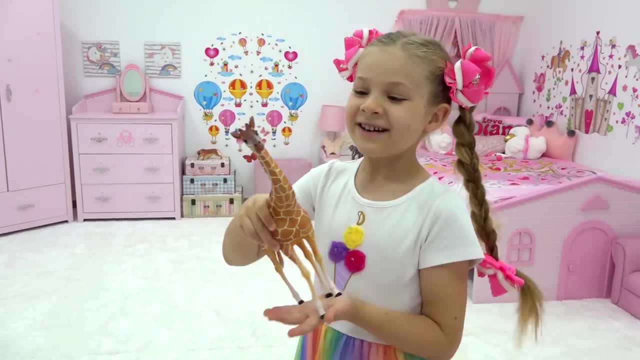 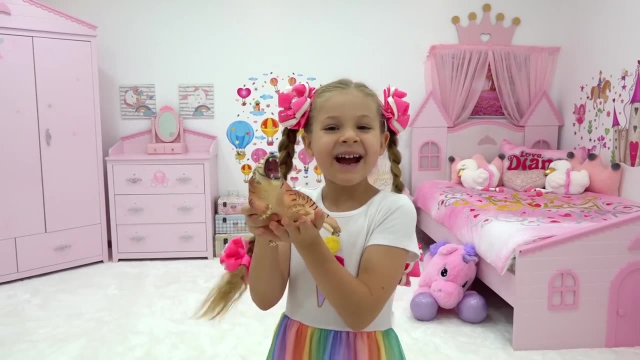 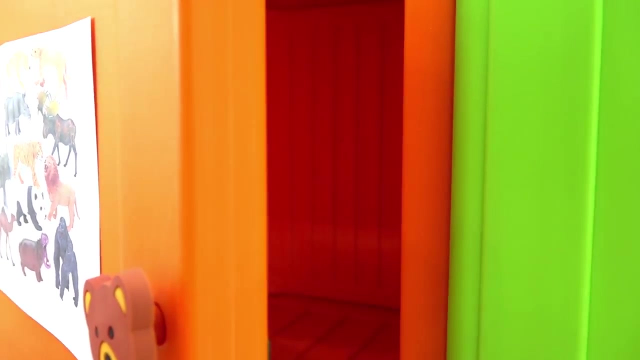 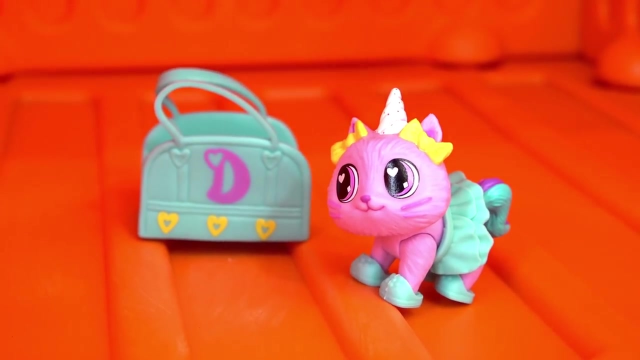 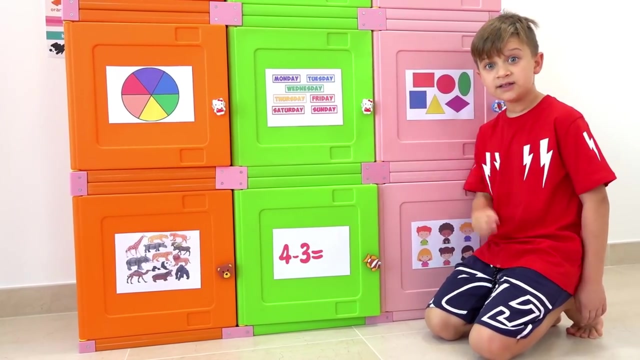 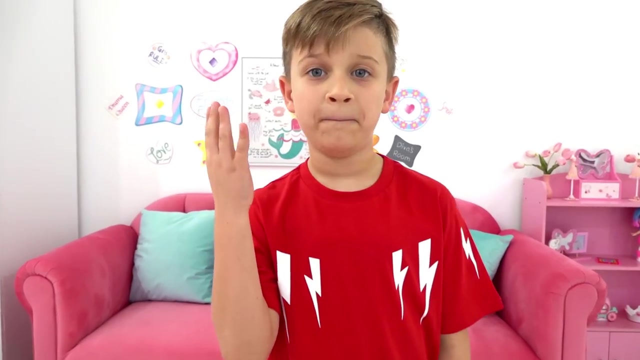 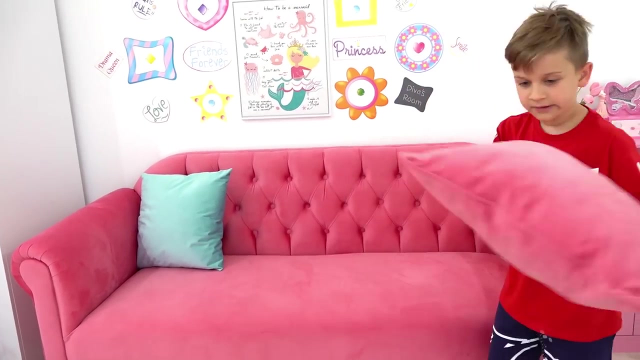 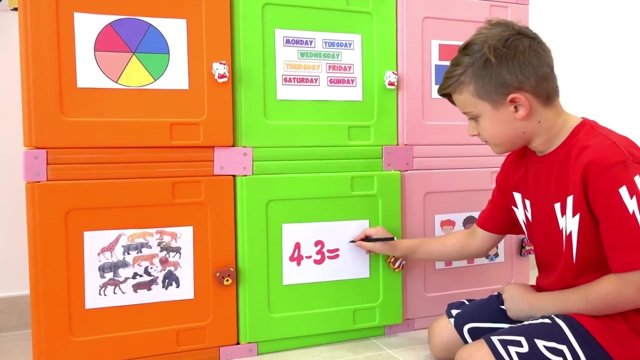 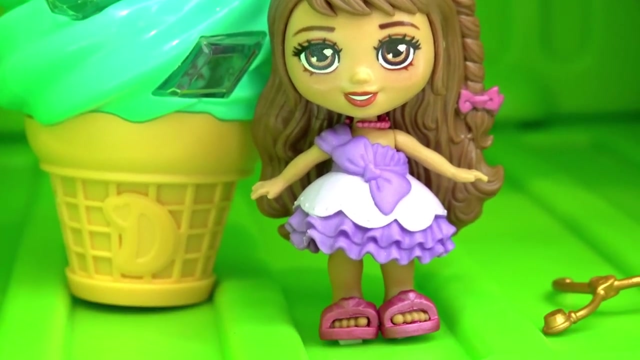 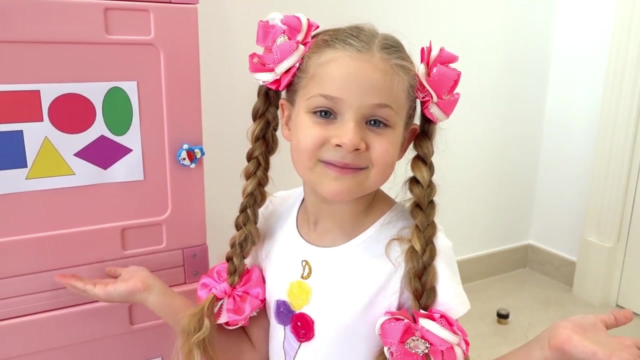 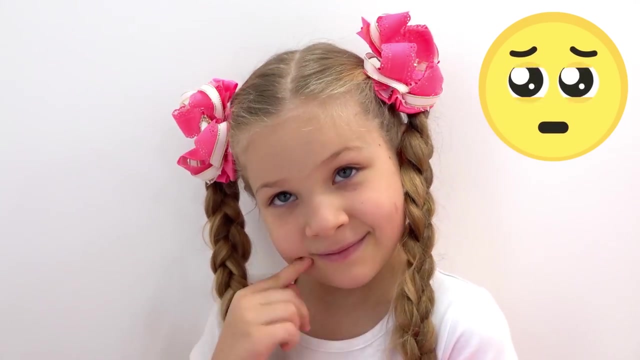 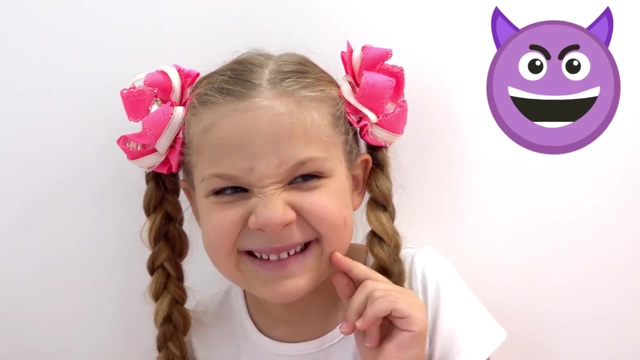 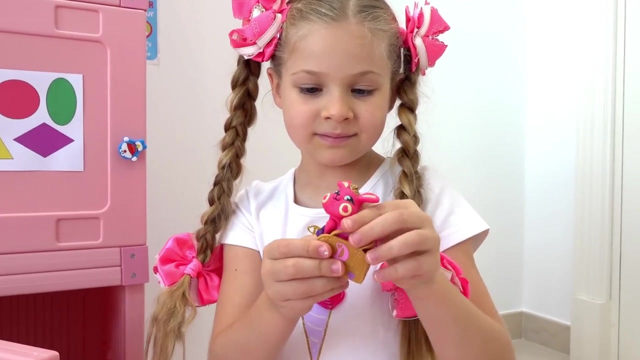 turtle, giraffe, elephant, tiger, fish, crocodile, cuckoo. four minus three. hmm, okay, we have four pillows, four minus three. one, two, three, equal one. okay, two, three, Ya Ho, nice girl. emotions: happy, sad, angry, shy, sleepy, crying, surprise, Sneaky, Upset, Mrs Everyone. 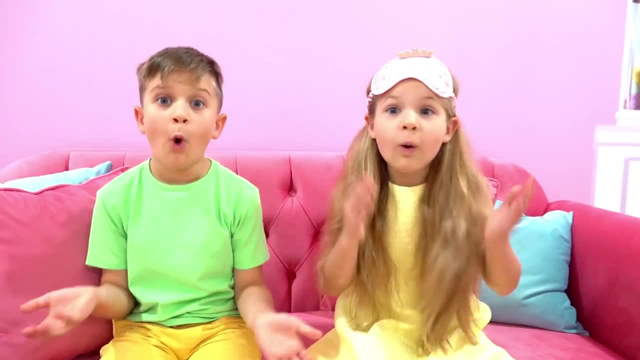 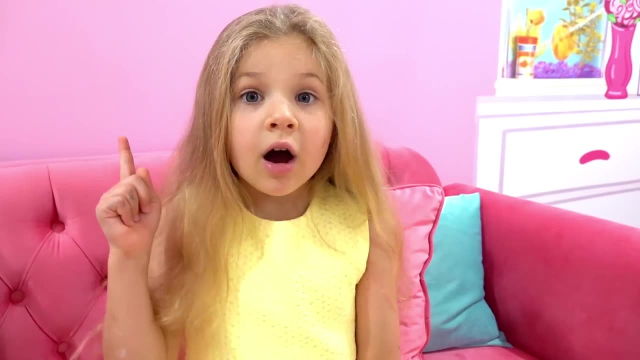 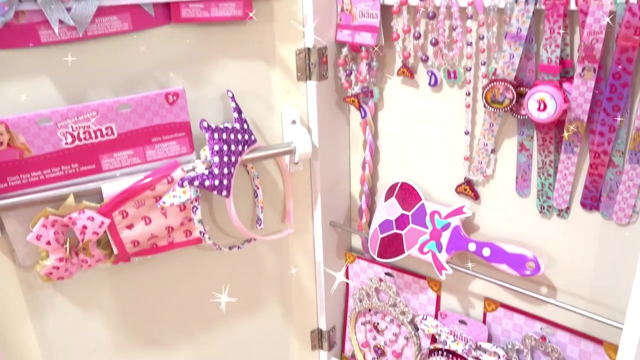 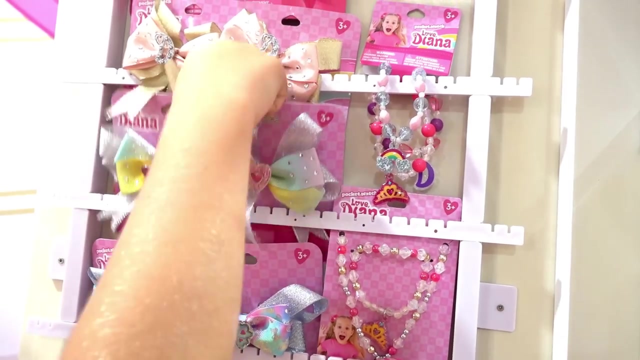 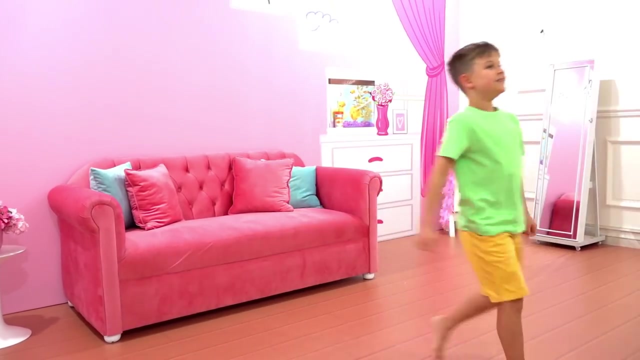 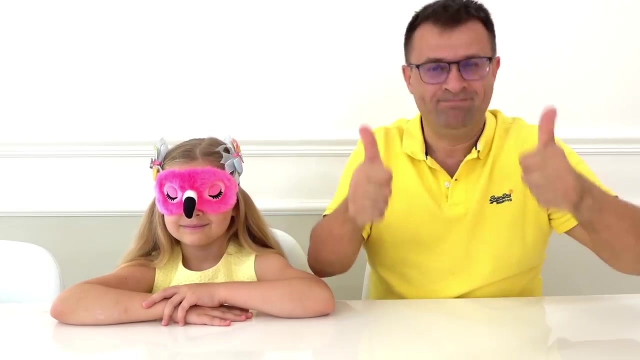 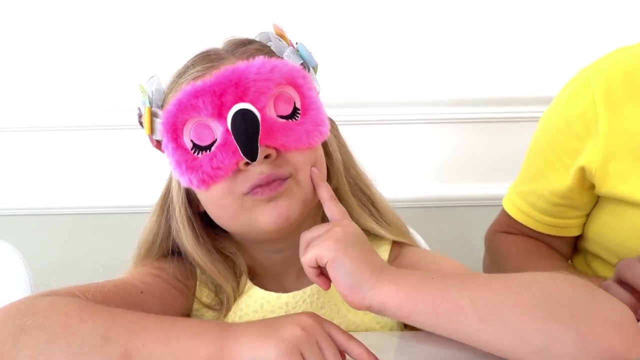 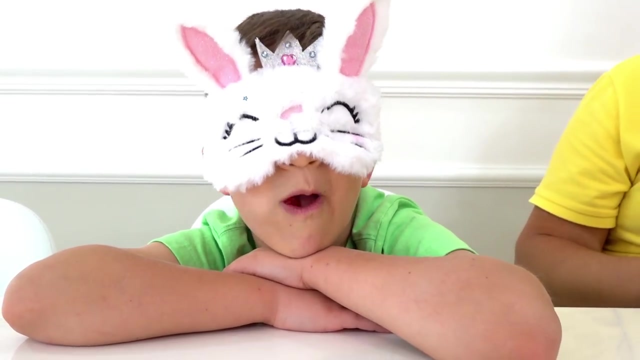 I know. Today we learn the senses: What Hearing, taste, smell, touch and sight. Wow, I need to be beautiful. Wow, Diana, you'll be first. What is this Cream? You're right, Tomato. I don't like tomato. 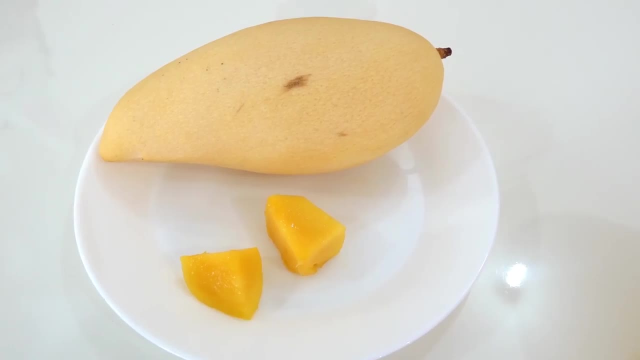 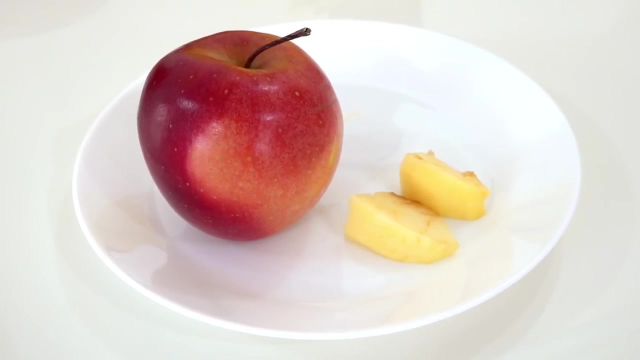 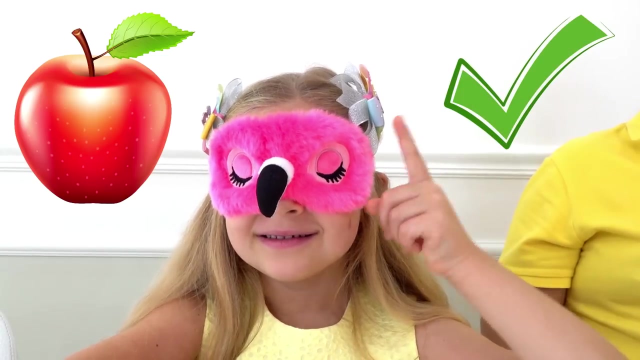 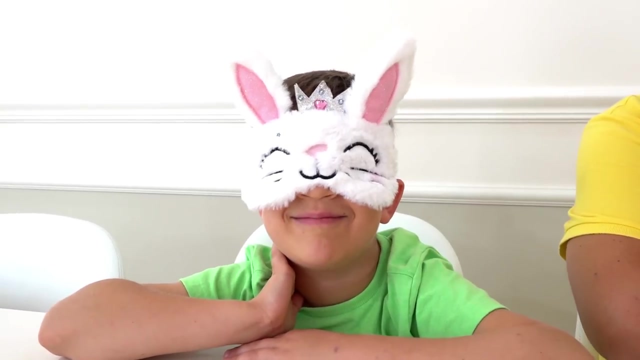 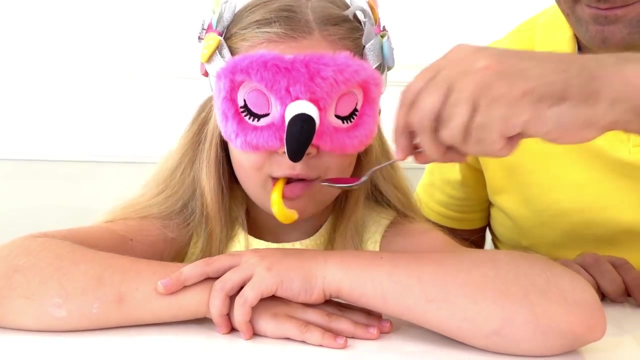 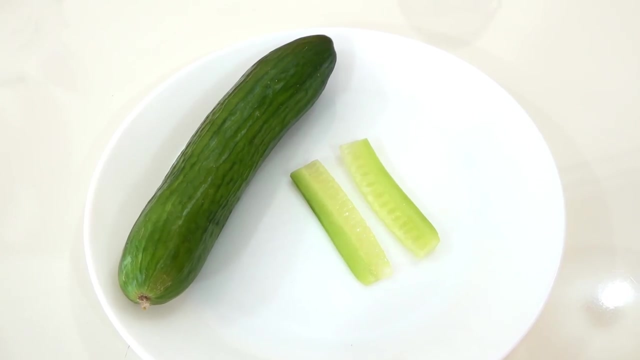 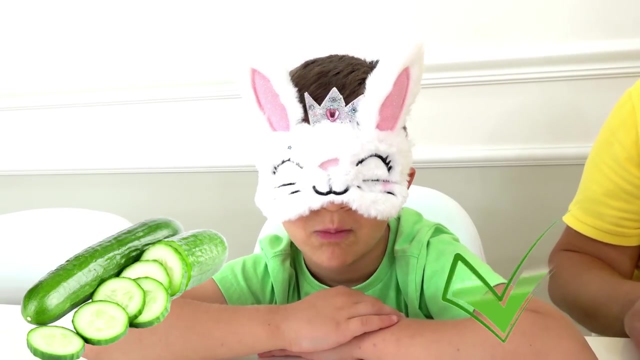 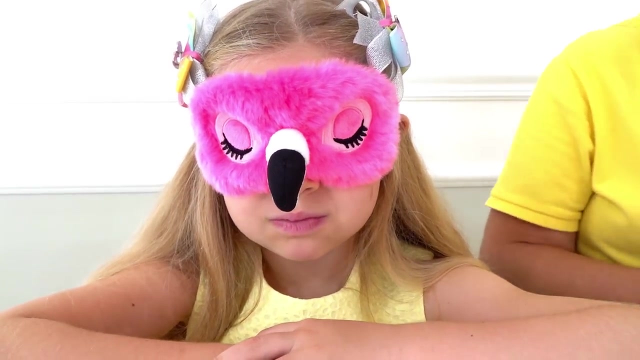 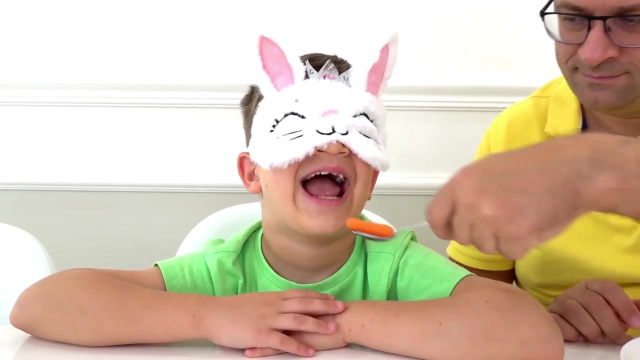 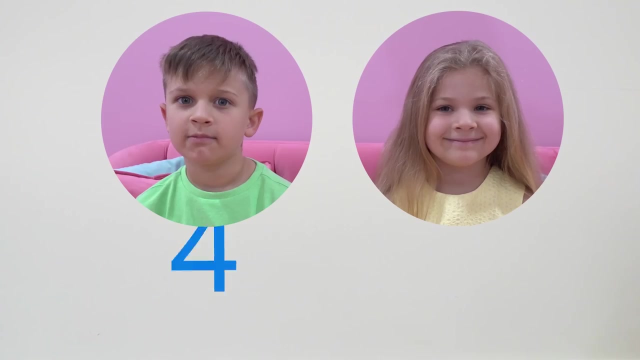 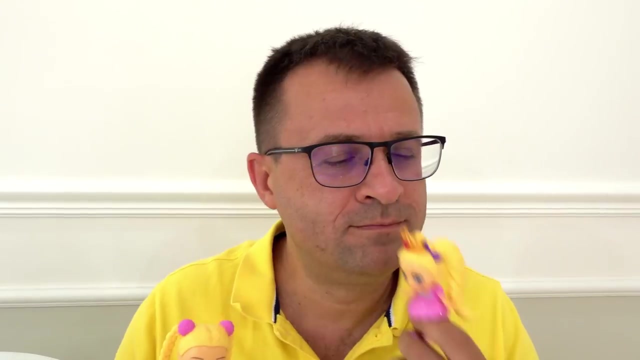 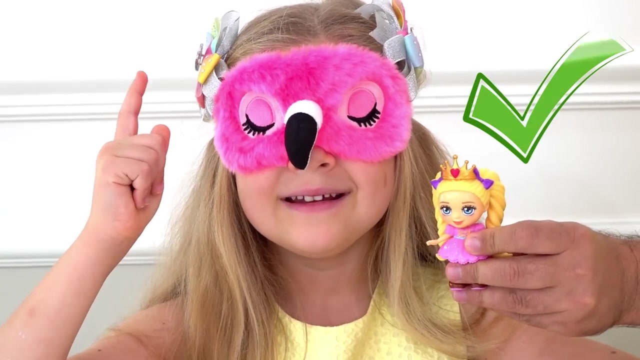 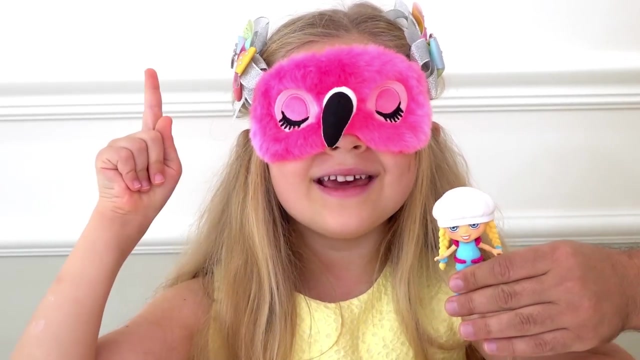 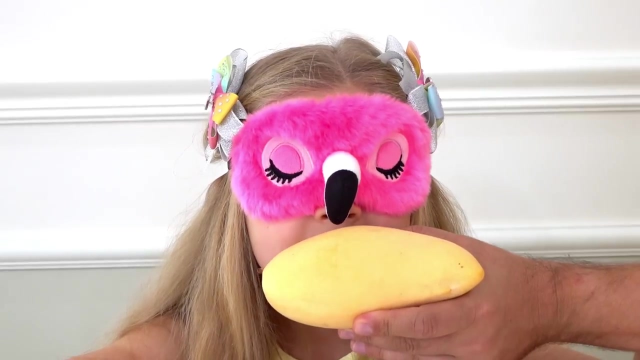 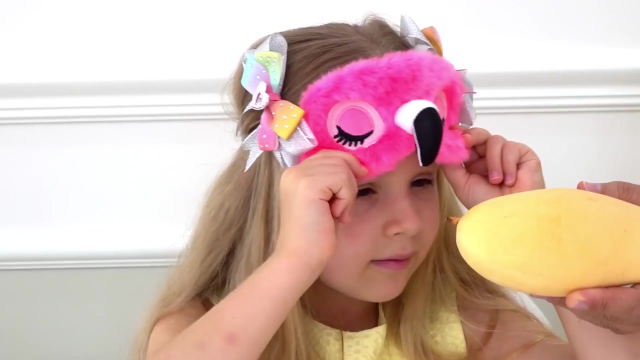 Blueberry Mango. Good job. Apple Kiwi, What Pepper? Super Cucumber, Tomato, OK, Carrot, Yeah, Next Smell, Learn, smell this doll. Strawberry, Cherry, Cotton candy Strawberry Mango. 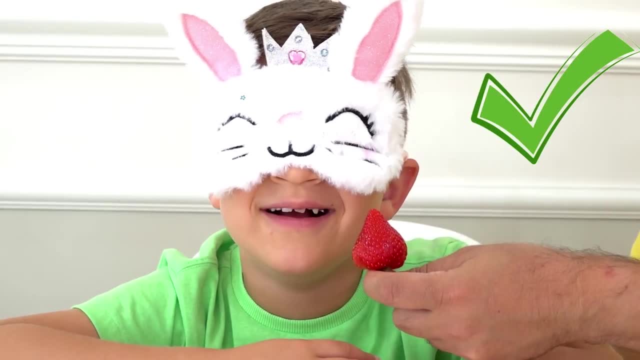 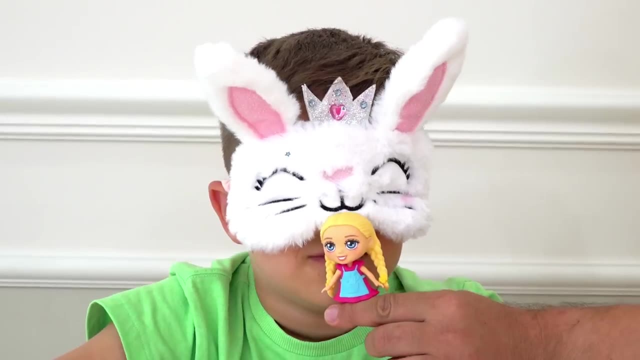 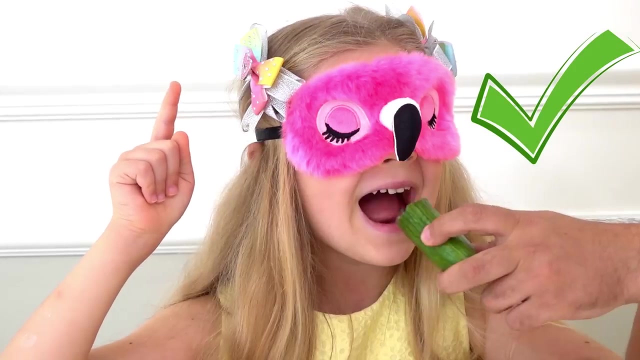 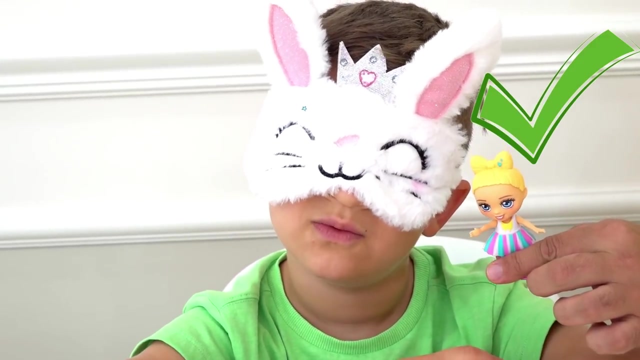 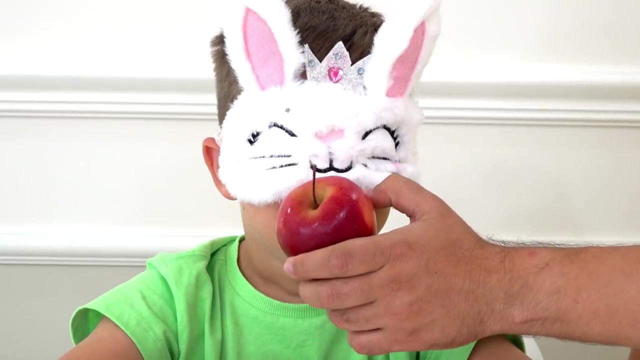 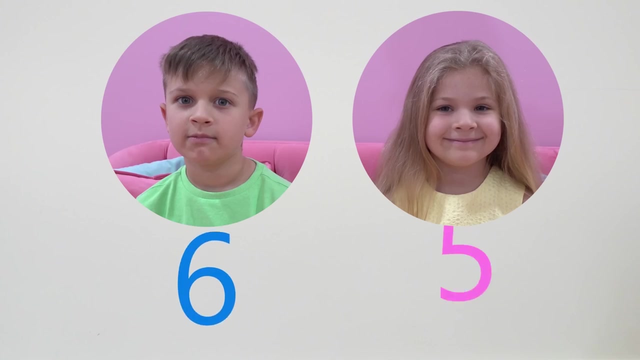 Strawberry, Strawberry, Strawberry, Cherry, Cherry. Apple, Apple, Apple Cucumber. Cucumber. Cucumber Smells like flowers, Smells like flowers. Vanilla, Super Diana, Apple, Apple, Apple Next Touch, Next Touch. 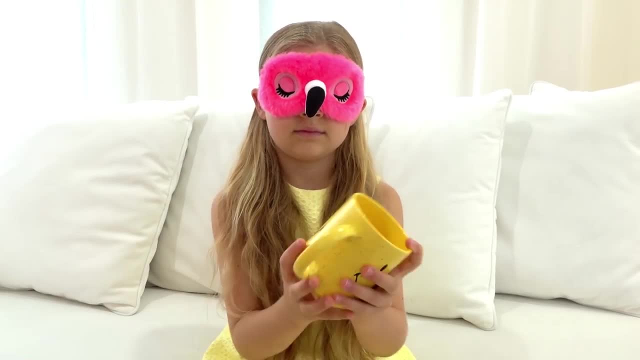 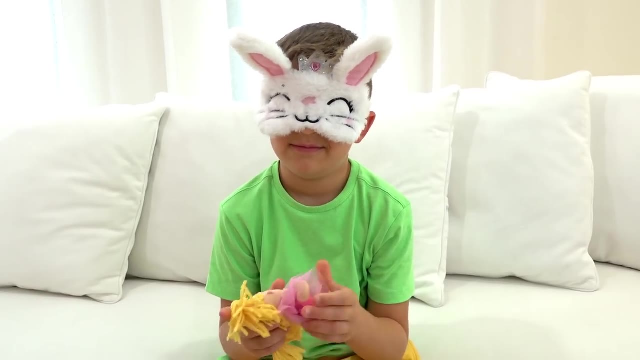 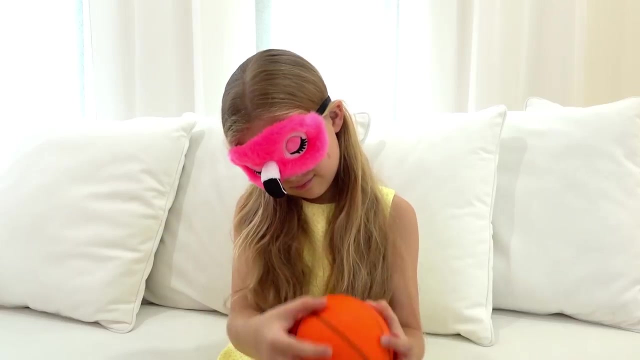 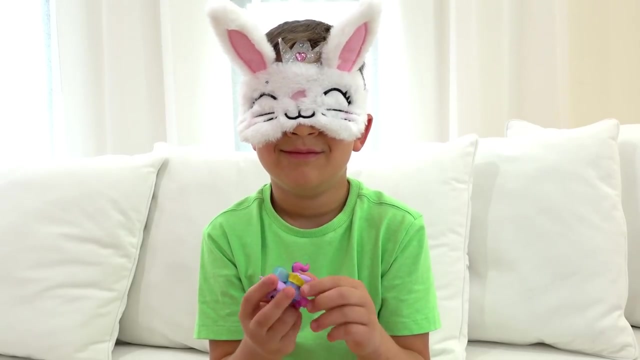 I'm ready, I'm ready. This is cat, This is cat, This is cat. Love Diana doll. Love Diana doll. estrella Roundա red people. I'm really excited. BOLO spon Spectacle Jabber. 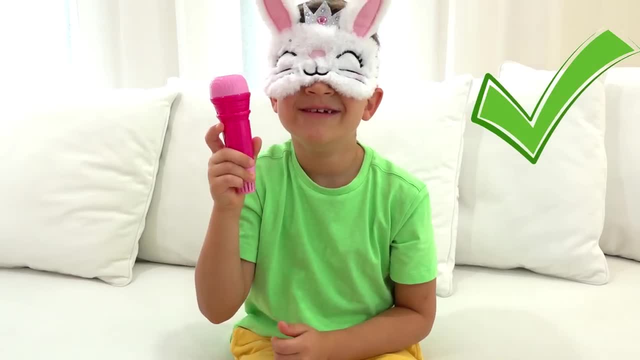 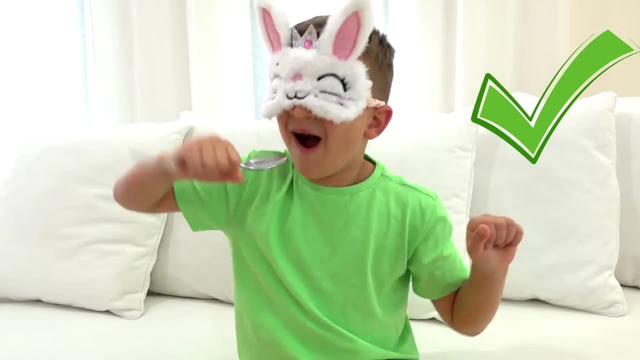 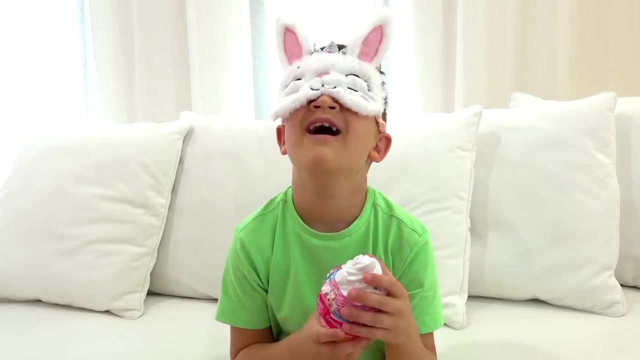 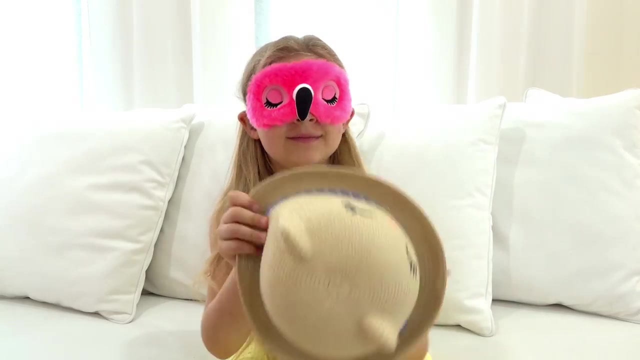 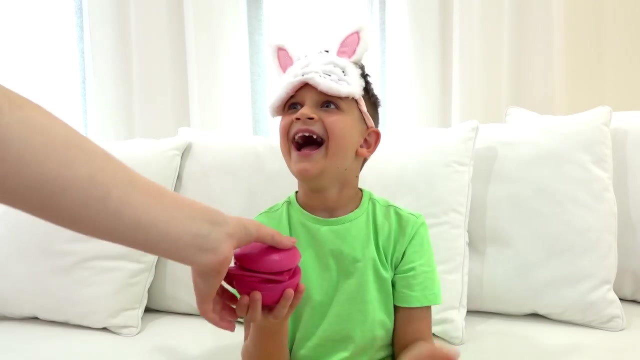 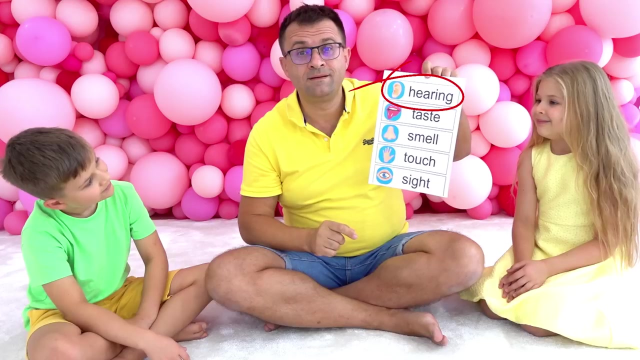 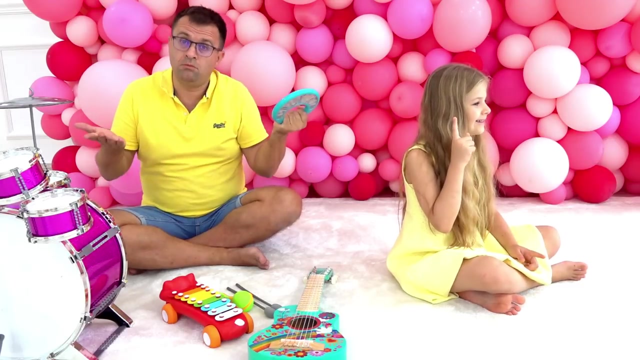 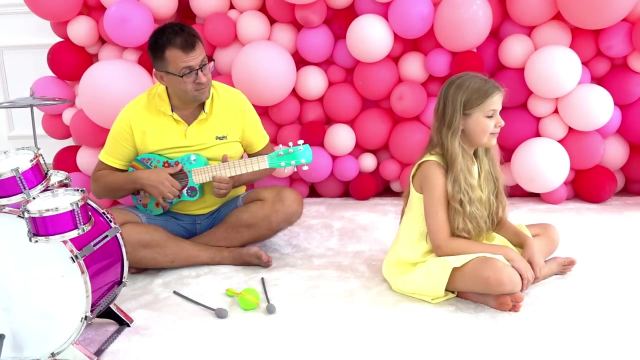 pr w Who Stream? Do u do? ooooo, do me transparency. The animals Love Diana. ice cream Hat, Pink burger Hearing. Diana, are you ready? Yes, Ice cream, Yay, Caterpone, Yay, Right Guitar. 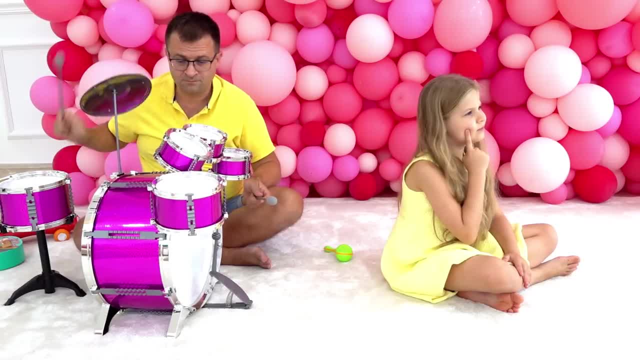 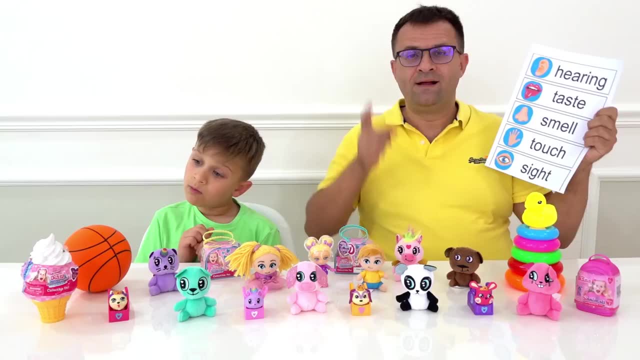 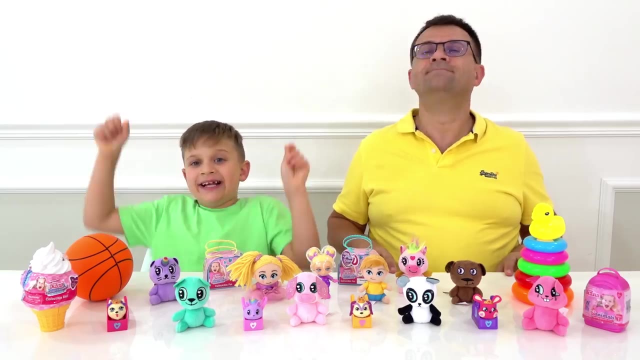 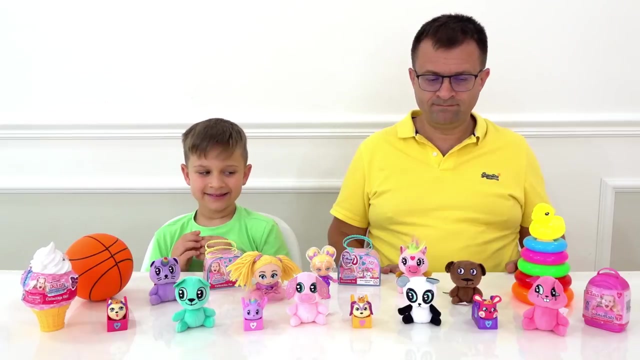 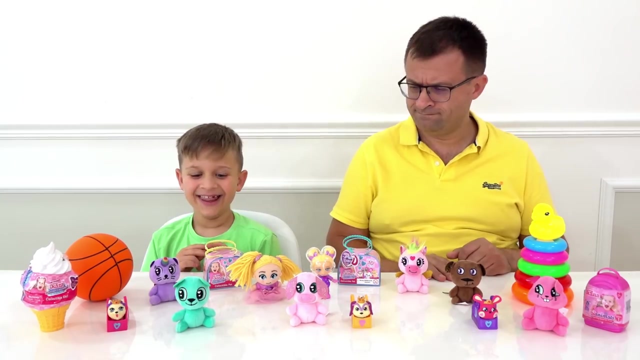 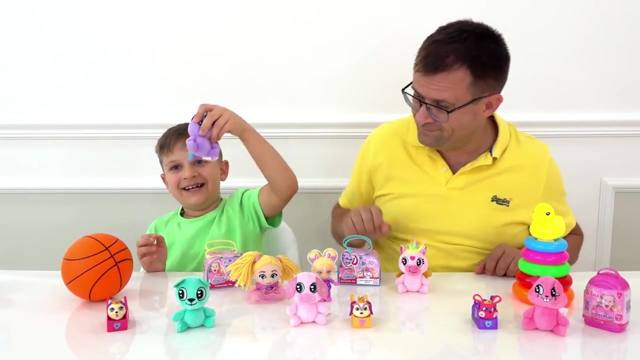 Right Dance. Yay, What are we doing? Right? Last one: Wow, Are you ready? Yes, Please find toys Roma. Please find pink basket, Panda Ice cream. Yes, Brown beer, Coco, pipico, Oilers toys. 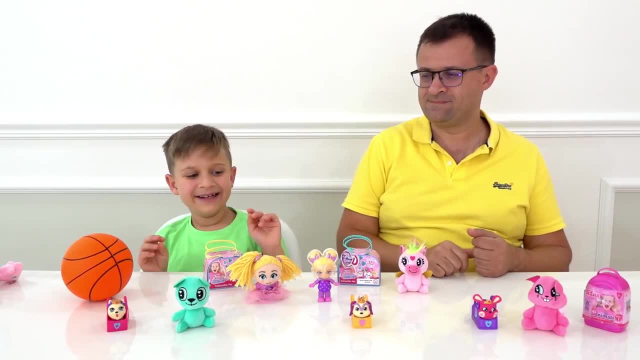 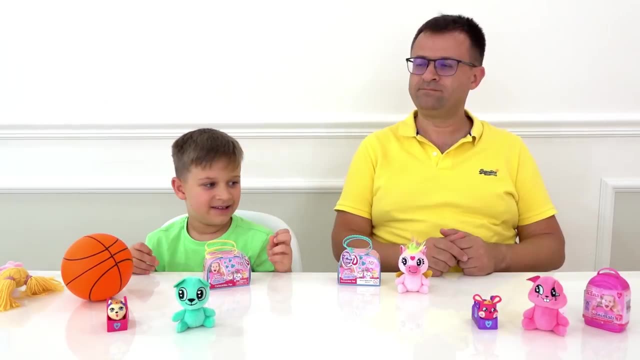 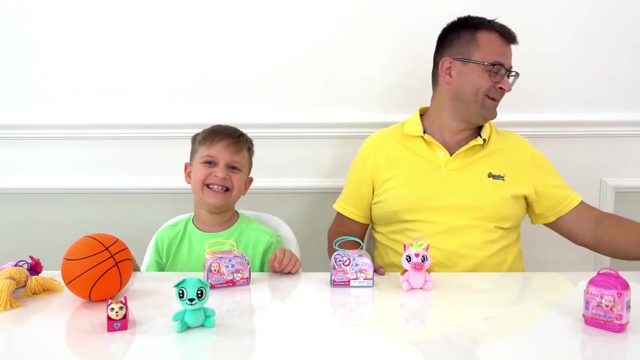 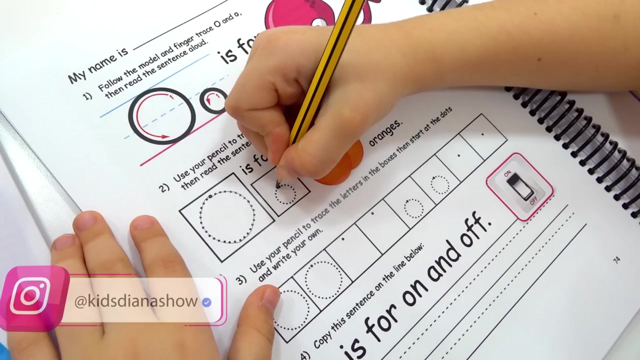 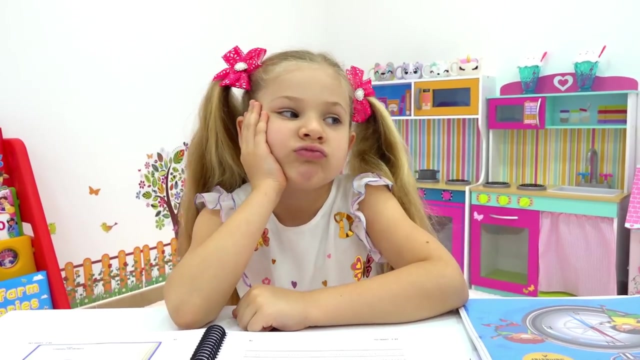 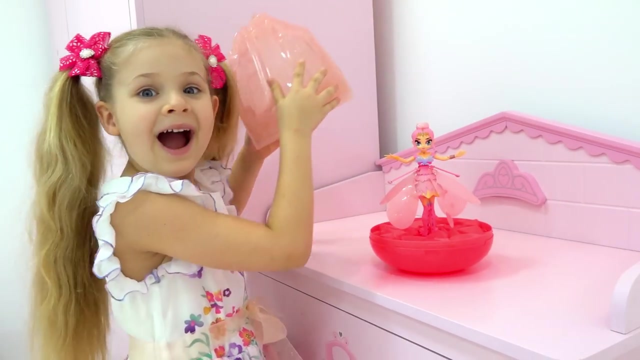 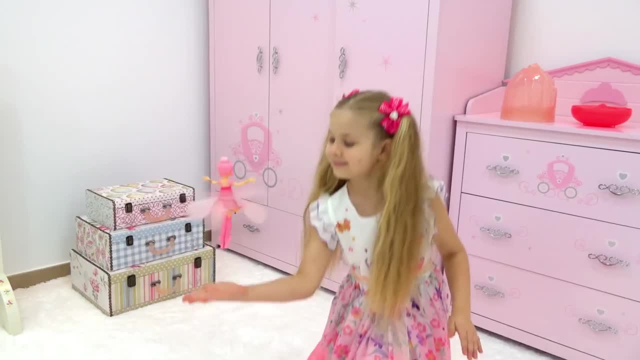 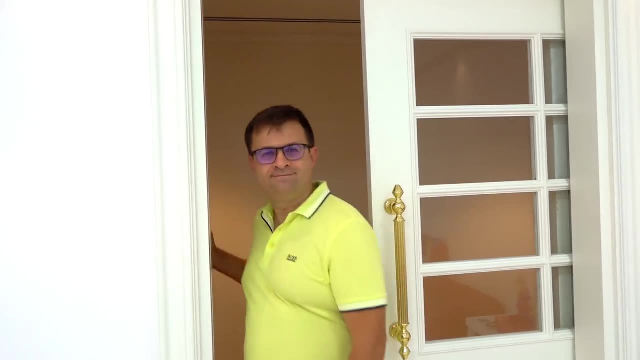 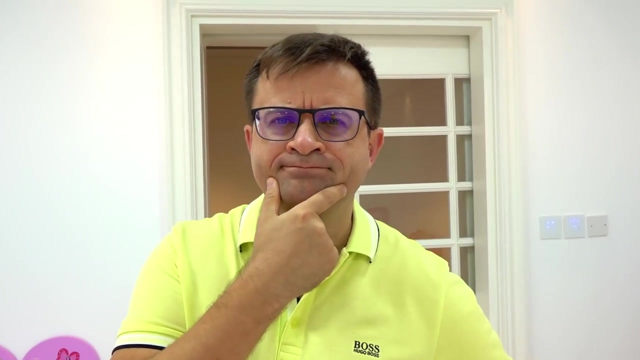 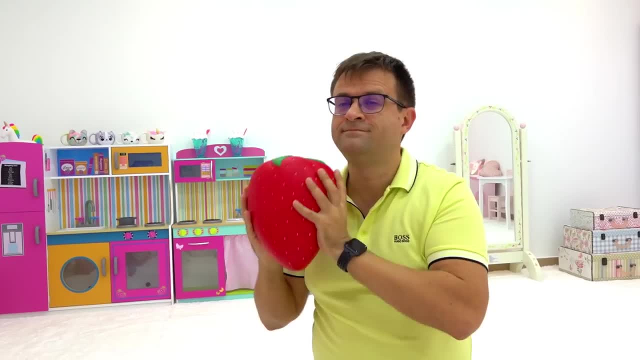 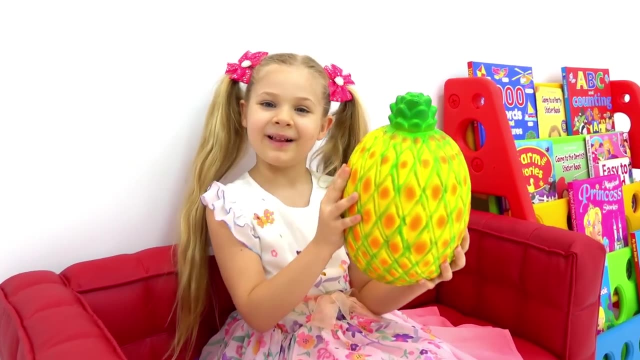 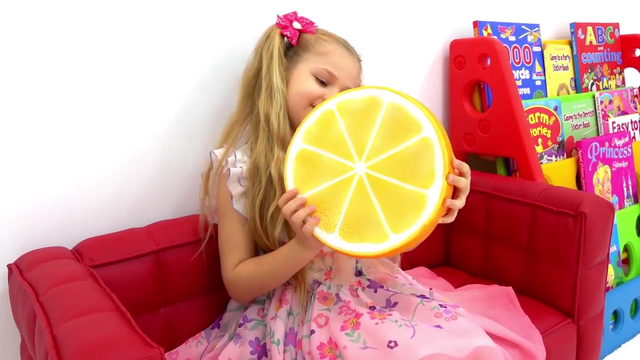 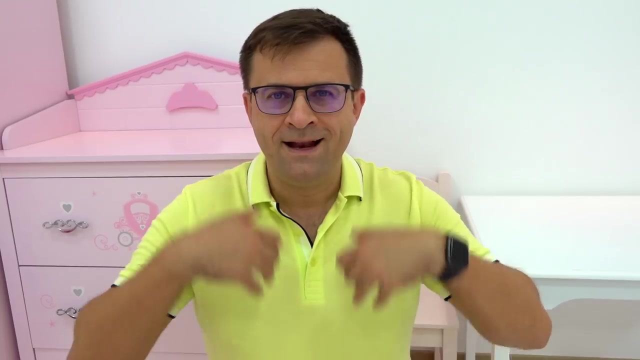 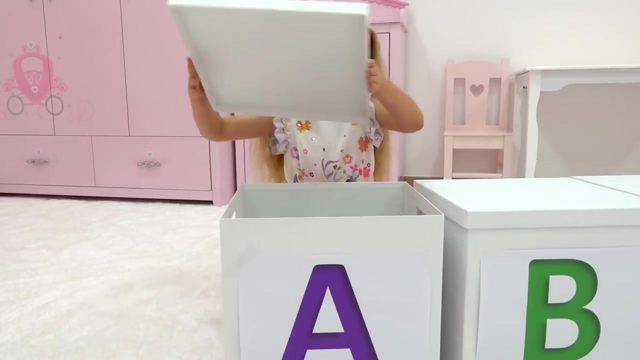 Yeah, What fruit is it? Strawberry, Strawberry, Pineapple, Pineapple, Watermelon, Watermelon, Orange, Orange, Peach, Peach, Super. Come on, come on Learning letters A, A, A, balloon A. 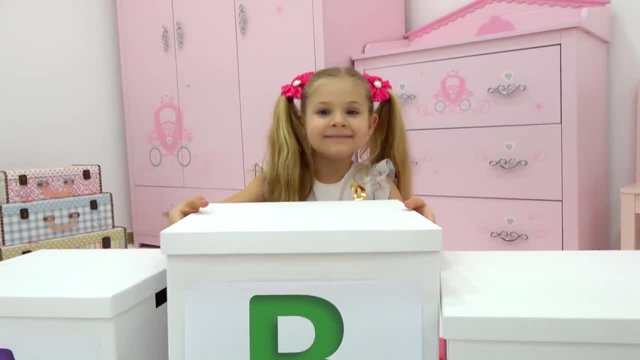 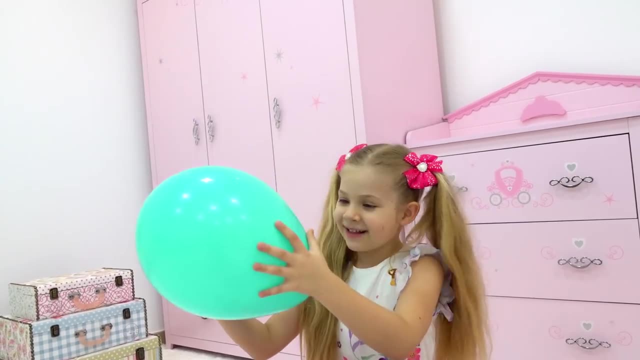 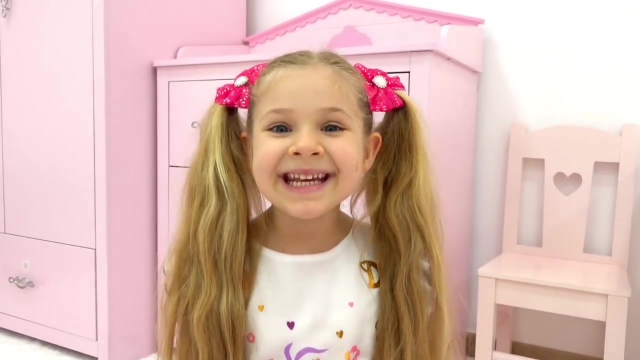 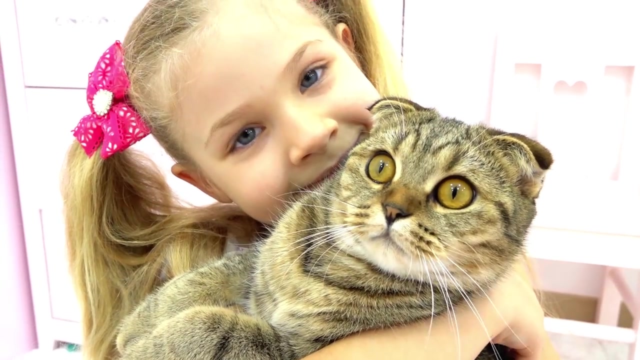 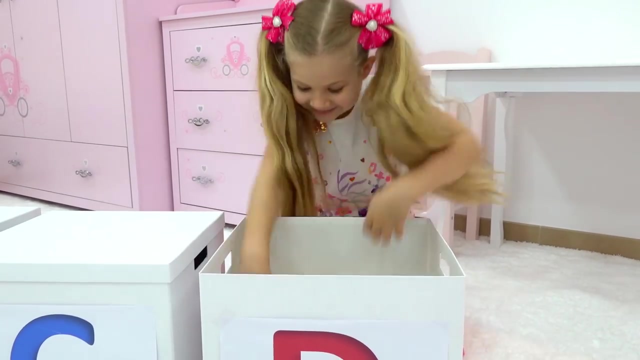 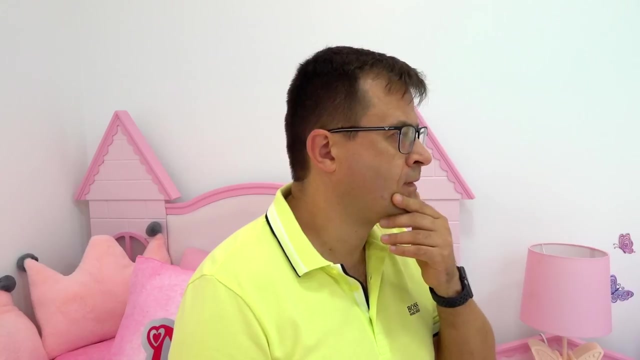 A, A, B, B. Balloon. Balloon One: Two, Yeah, C, C, C, Kid, Kid, Kid. Maybe Diana C Dance Very good, Learn animals. C, C, C. 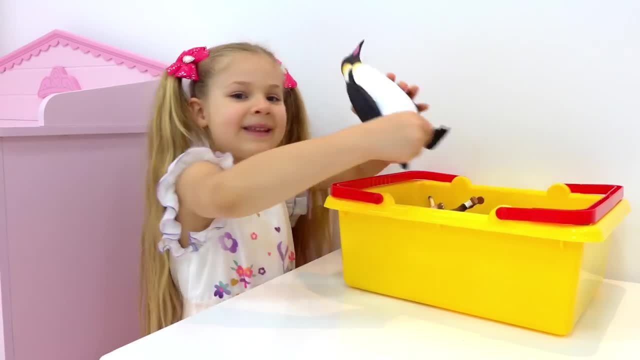 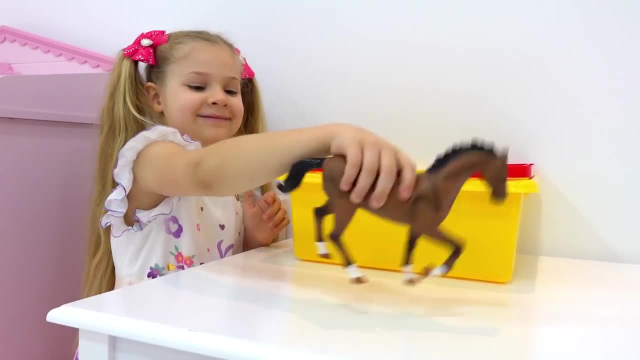 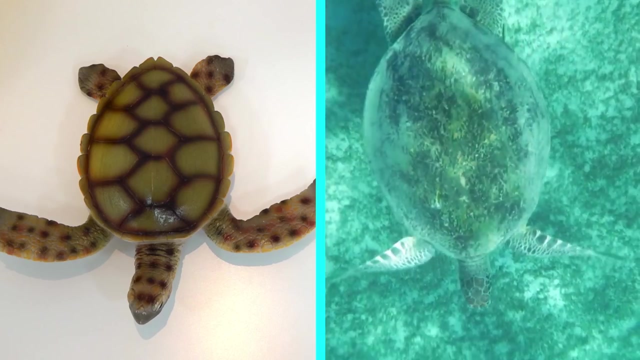 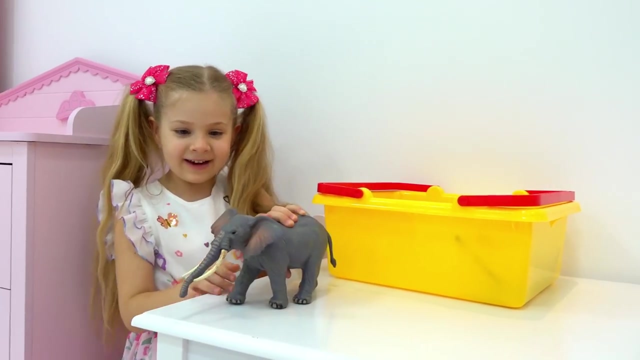 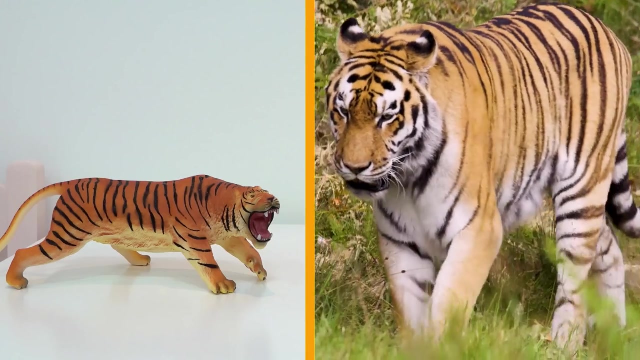 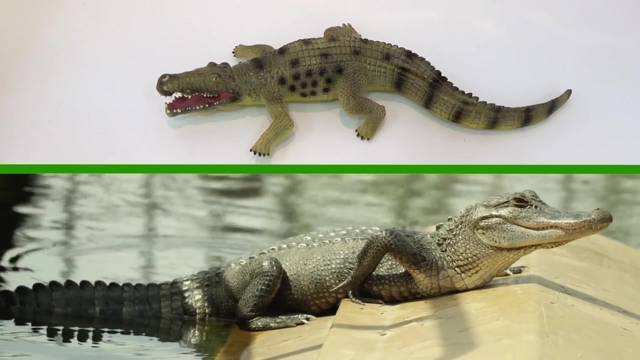 Wow, Pinguin, Pinguin, Cute Horse, Whee Whee Turtle. Wow, Wow, Kangaroo, Cool Elephant, Amazing Dagger Alligator. Wow, Wild Bear, Wild Bear, Wild Bear. 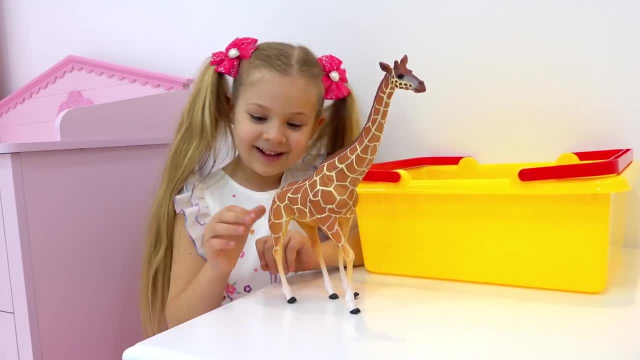 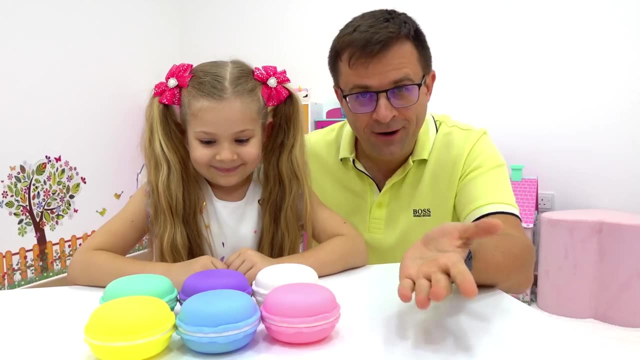 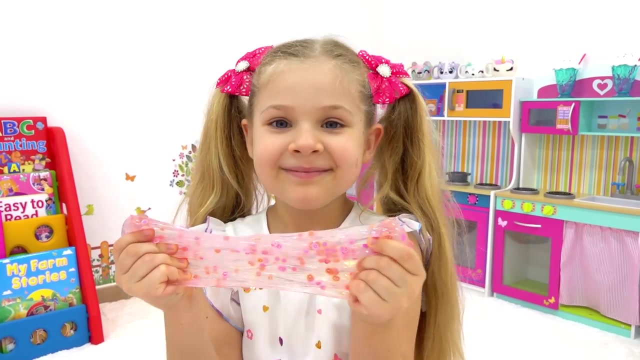 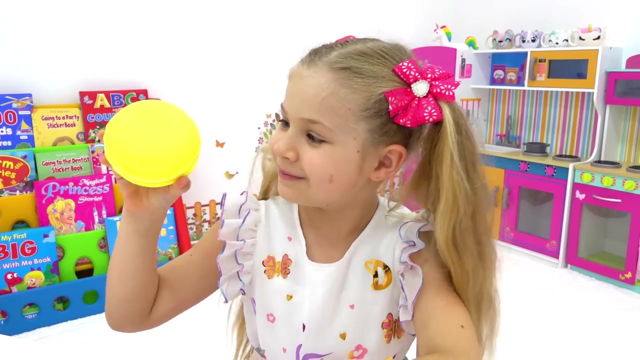 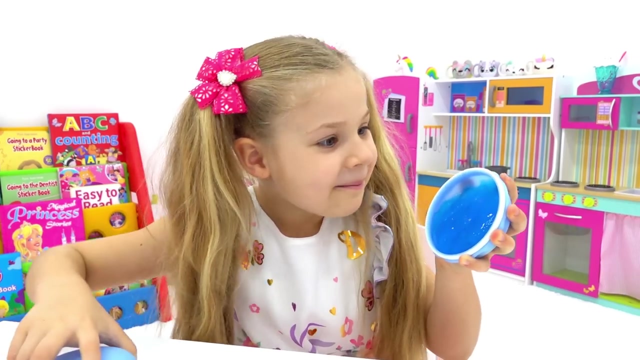 Yeah, Yes, Wild Bear, Wild Bear, Wild Bear. Your colors, Wow, Blue, Yellow, Pink, Blue, Green, Purple, White, Super, I like color slime. Next we learn the sizes: Blue, Blue, Blue.